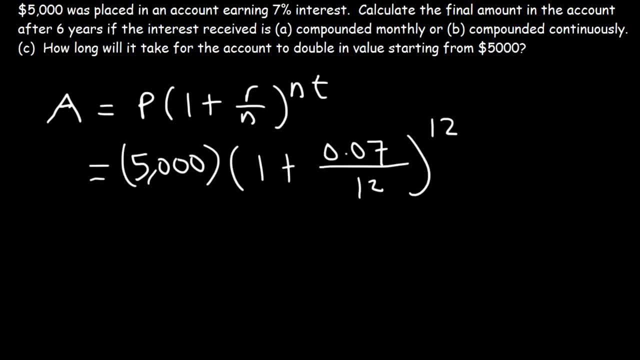 There's 365 days in a year. So if you hear the word daily, n is 365.. Weekly n is 52.. Quarterly n is 4.. Semi-annually n is 2.. Annually n is 1.. 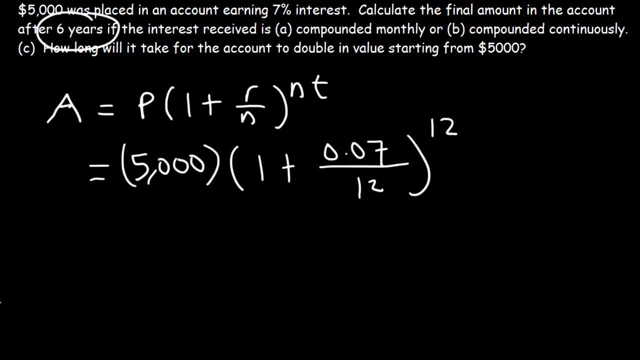 Now we want to find out how much money will be in the account after 6 years. t is the time in years, So now all you need to do is just type this in your calculator, exactly the way you see it, And you should get $7,600. 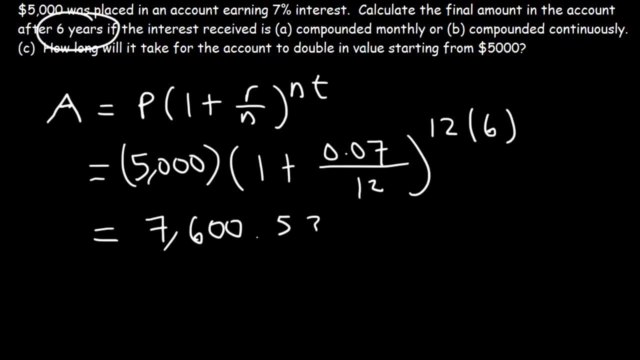 And you should get $7,600. And 53 cents. So it's $7,600. And 53 cents. Now what about part b Compounded continuously? How much money will be in the account if it's compounded continuously? 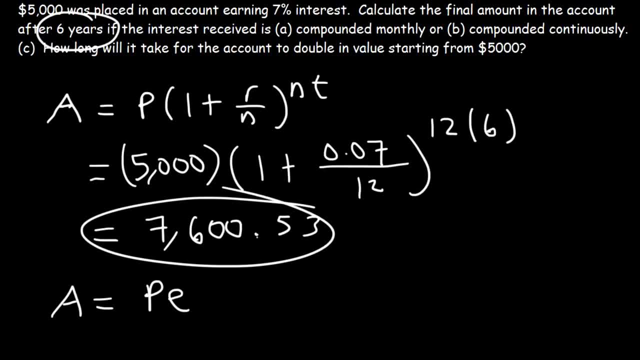 You need to use a different equation. a is equal to pe. raised to the rt, p is 5000.. r is .07.. And t is 6.. So it's 5000 e raised to the .07 times 6.. 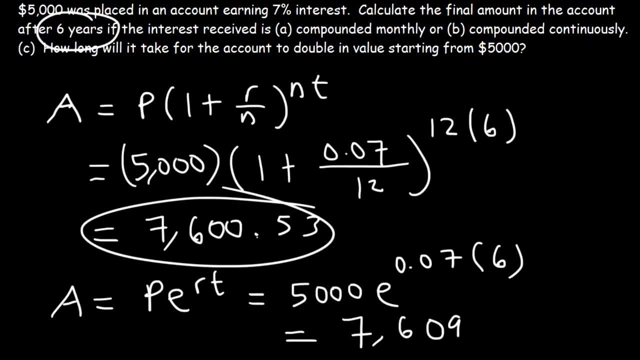 And this is equal to $7,609.81.. So it's very close to this answer, But when it's compounded continuously the amount should be a little bit higher. Now part c: how long will it take for the account to double in value, starting from 5000?? 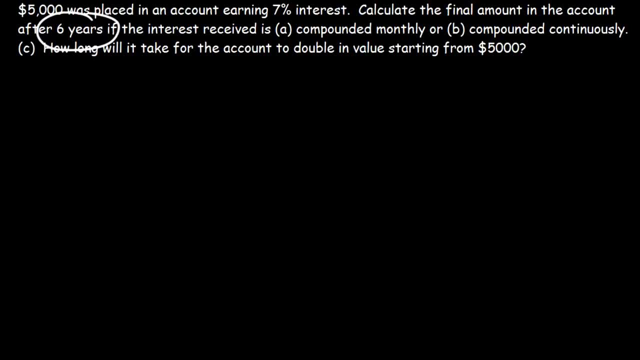 Now, the only thing that I didn't mention for part c is if it's compounded monthly or continuously. So let's go with part a. Let's say that it's compounded monthly. If we're looking for how long we need to find the value of t. 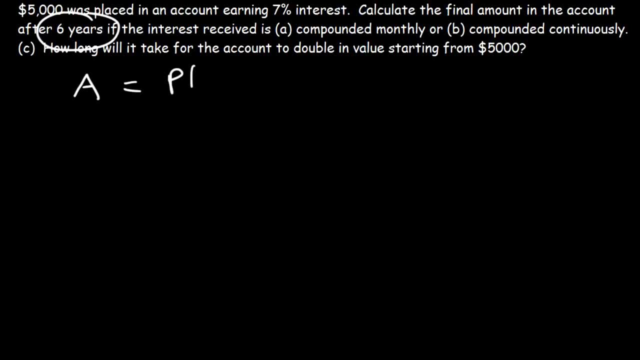 So let's rewrite the equation: a is equal to pe1 plus r over n raised to the nt, So the principal is 5000.. Now the account is going to double in value. So if you multiply 5000 by 2, it's going to be 10,000. 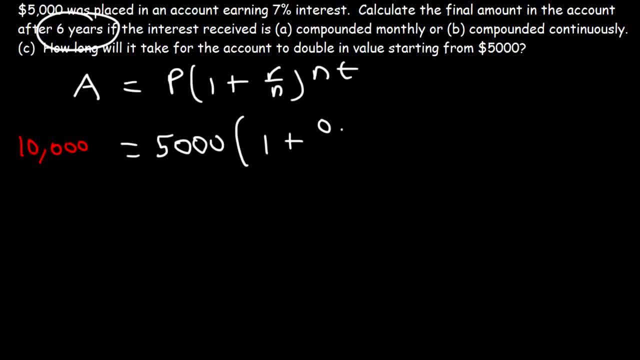 r is still .07.. If it's compounded monthly, n is 12.. And we've got to find t this time. So the first thing we need to do is divide both sides by 5000.. 10,000 divided by 5000 is 2.. 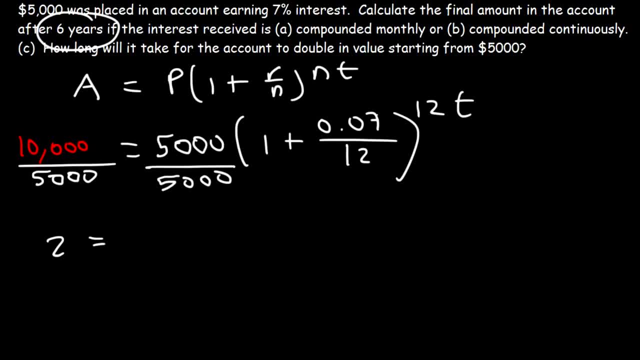 Now what I'm going to do is simplify this equation. I'm going to use this expression on the inside: .07 divided by 12 plus 1. That's about 1.00583.. And that's raised to the 12t. 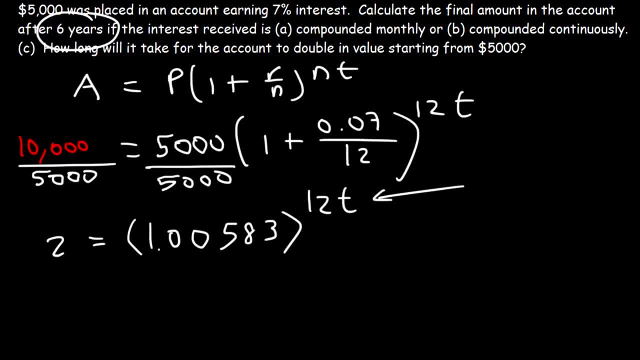 Now, anytime you want to solve for a variable that is in the exponent position, take the natural log of both sides. You can use a regular log as well. Once you take the natural log of both sides, you can move the exponent, In this case the 12t. 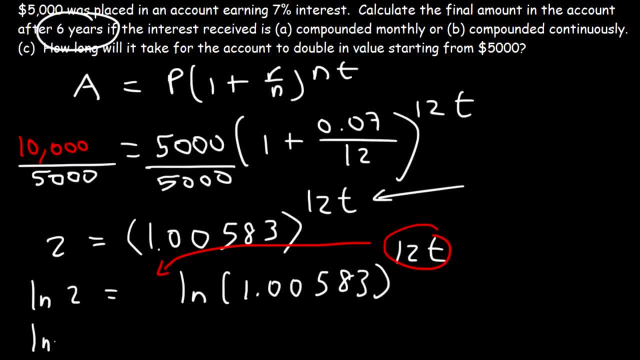 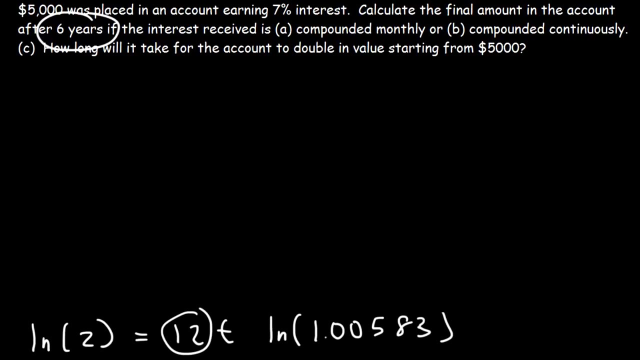 to the front, And so the natural log of 2 is equal to 12t times the natural log of 1.00583.. So now, at this point, we just need to do some algebra and then we can get the answer. So let's divide both sides by 12. 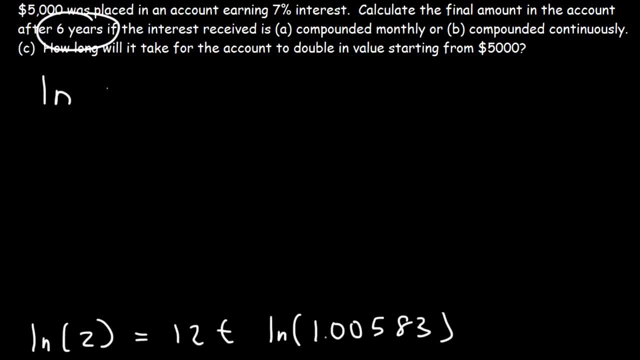 and ln of that number. So ln2 divided by 12 times the natural log of 1.00583.. That should equal t And your calculator. if you're not getting the right answer, make sure you enclose this in parentheses. That should help. 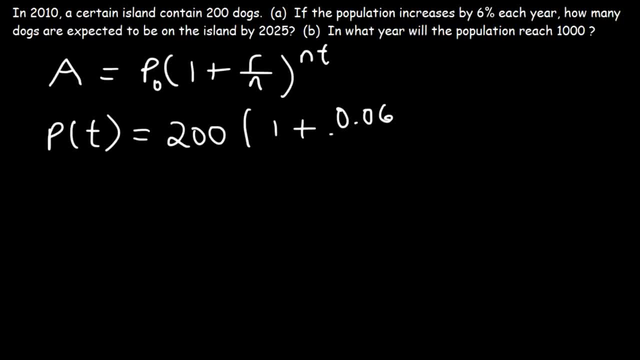 t is equal to zero because in that year we have the initial population, which was 200. so in 2025, 15 years later, t is going to equal 15. so we need to find the 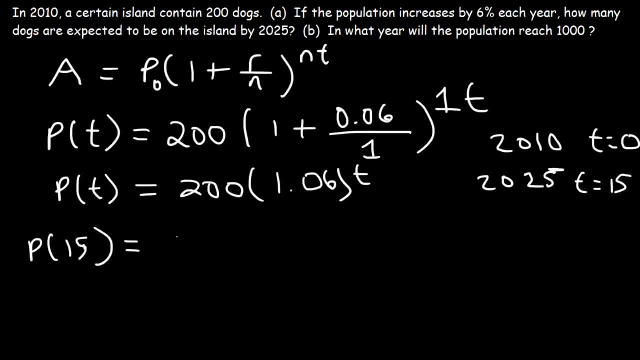 population, which is 15. so it's 200 times 1.06 raised to the 15, and so that's going to be 479.3. so that's going to be about 479 dogs in the year 2025. Now, in And what year will the population reach 1,000?? 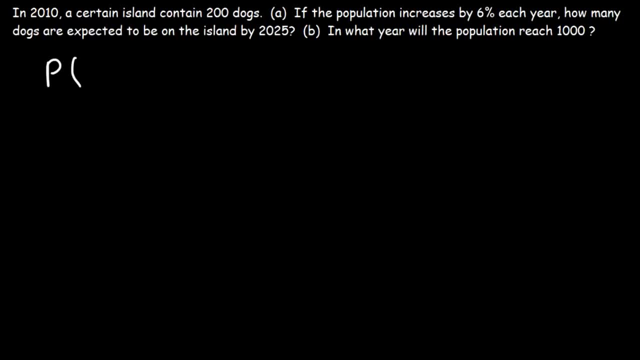 So let's start with this equation: PFT is equal to 200 times 1.06 raised to the T. So PFT, let's replace it with 1,000. And our goal is to solve for T. So the first thing that we need to do is we need to divide. 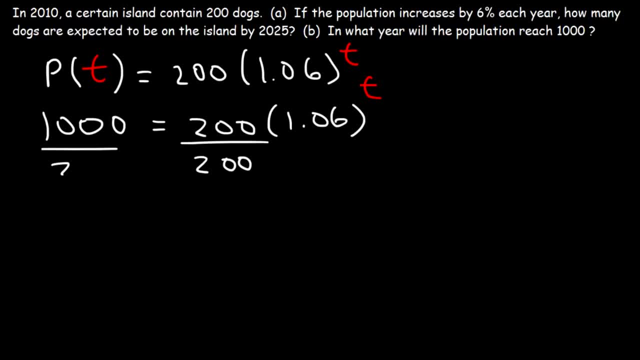 both sides by 200.. 1,000 divided by 200 is 5.. So now what we need to do is take the natural log of both sides. So the natural log of 5 will be equal to the natural log of 1.06 raised to the T. 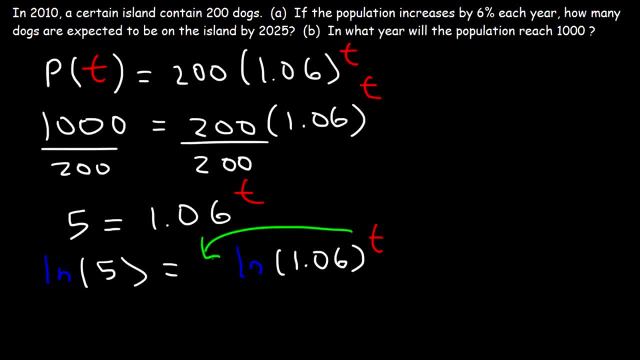 So now let's move this variable to the front. So LN of 5 is equal to T times LN of 1.06.. So in order to solve for T, we need to divide both sides by LN 1.06.. So it's going to be the natural log of 5 divided by the natural log of 1.06.. 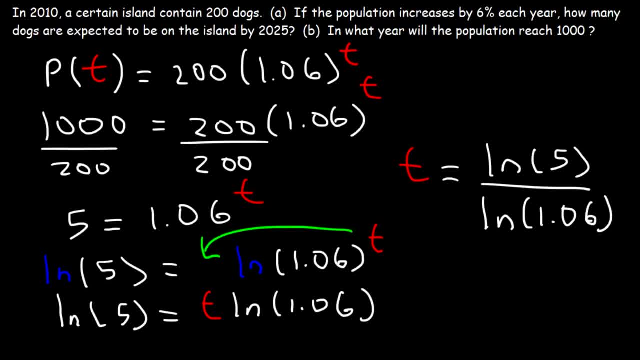 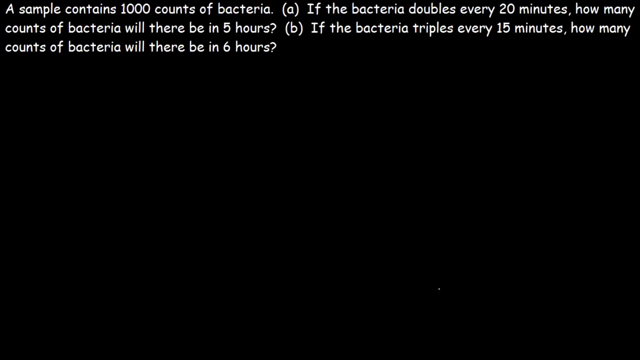 Okay, So that's it Bye. 2,019.. Time in mass: 12,200.. menos 10.. 3,635. 1,000. 1,000. 1,000.. Yeah, sometime between 2037 and 2038.. A sample contains a thousand counts of bacteria. 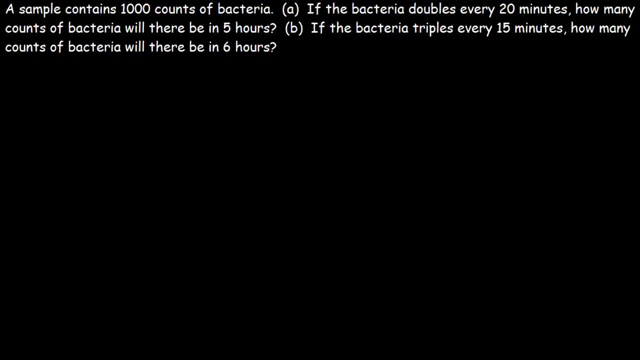 If the bacteria doubles every 20 minutes, how many counts of bacteria will there be in five hours? So we need to write an equation. So this is going to be the population of bacteria. Initially we have a thousand and it doubles, so we're going. 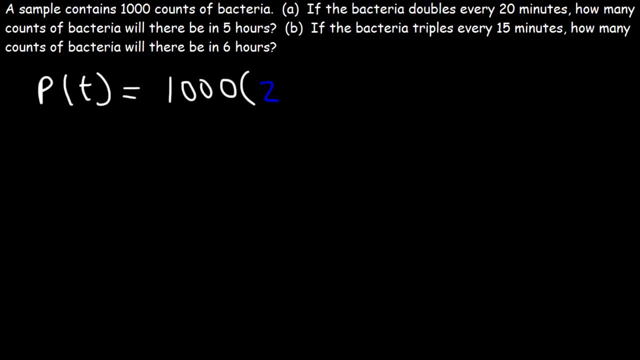 to put a 2. It doubles every 20 minutes. so you can write the equation two ways. If you want to beI mean if you want T to be in minutes, it's going to be T over 20, because every 20 minutes is going to double If you plug in 20, 20 over 20 is. 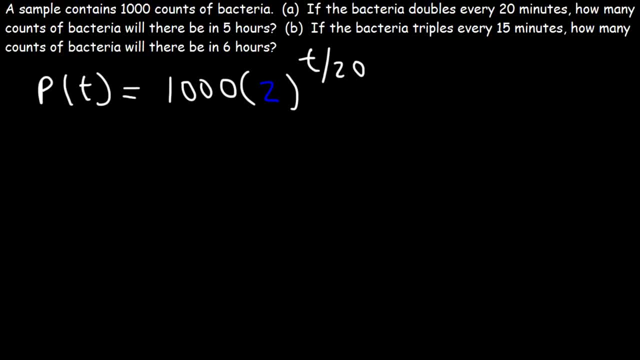 1. 2 to the first is 2, so it doubles. If you plug in 40,, 40 over 20 is 2.. 2 squared is 4, so it doubles twice, which is equal to 2. to 4.. So that's the equation if you want t in minutes, but we want to know how. 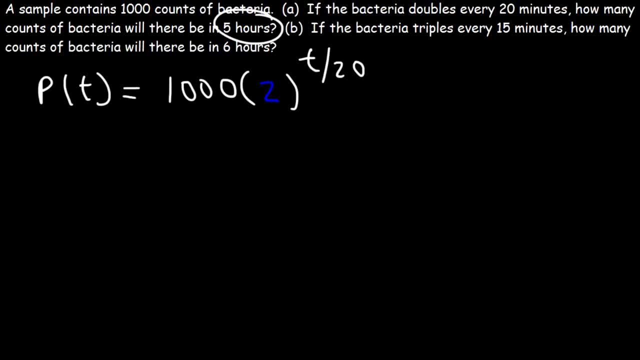 many bacteria or counts of bacteria. that's going to be in five hours, So we want t in hours. So if it doubles every 20 minutes, how many times does it double in one hour? Well, there's 60 minutes in an hour, and so there's three intervals of. 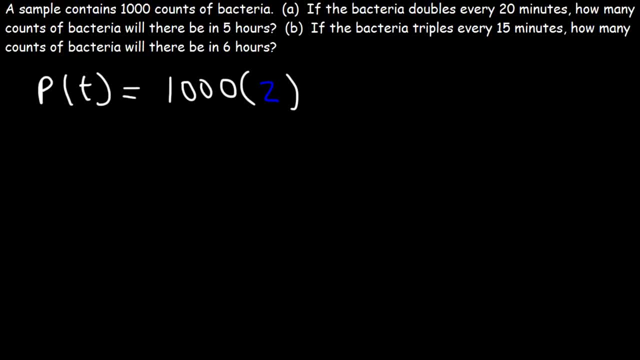 20 minutes within the hour. So if it doubles every 20 minutes, it's going to double three times in one hour. So we can write it as 3t, because if you plug in 1, 2 to the third is 8, which is 2 times 2 times 2.. It's doubling three times in. 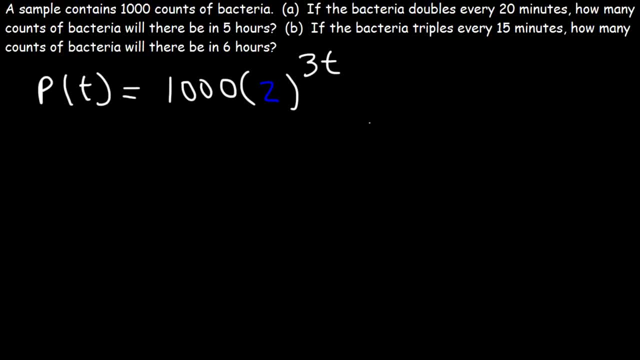 that single hour. So that's the equation that we need, where t is in hours. So now all we need to do is replace t with 5.. So if it doubles three times in one hour, it's going to double 15 times in five hours. So it's 2 to the 15 times 1,000, and it's going to be. 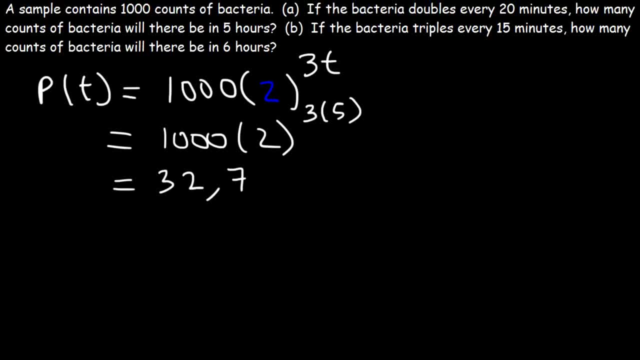 equal to a big number, 32,768,000.. Now what about part B? If the bacteria triples every 15 minutes, how many counts of bacteria will there be in six hours? Feel free to try this example. So let's begin. Let's write an equation for the population with respect to t. So